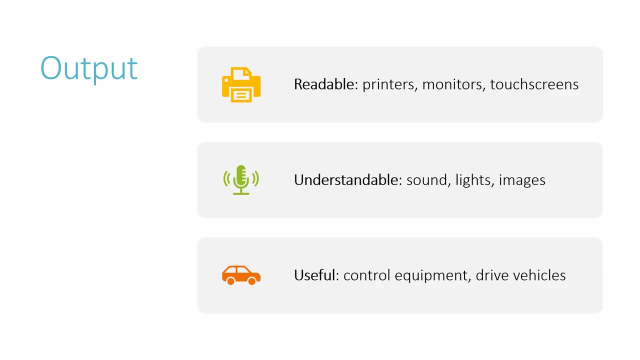 Output is anything that is produced by the computer which is useful to us as humans. It could be readable output, so that we can visually see it, or understandable in some other way, such as sound. Or it could be useful to us, for instance, controlling some kind of equipment: vehicle heater. 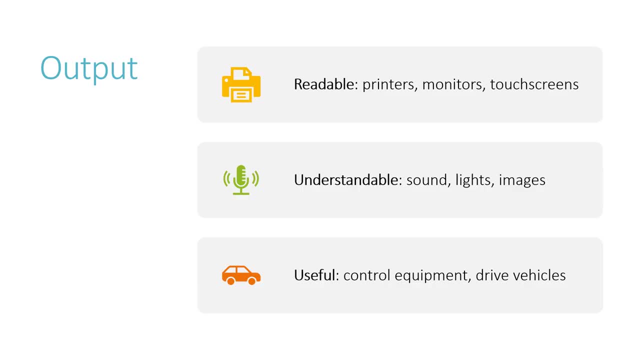 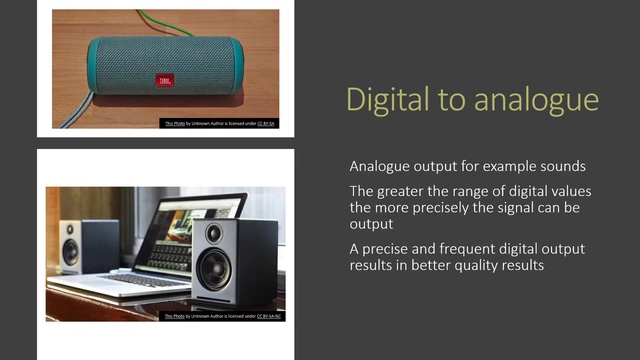 But in any case, all three of these types of output are important. They are something that we need as users. In the input lesson I talked about analogue to digital conversion, That is, turning the smooth analogue data of real life into number form. 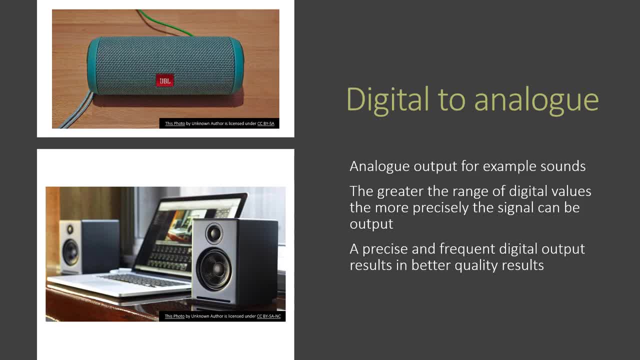 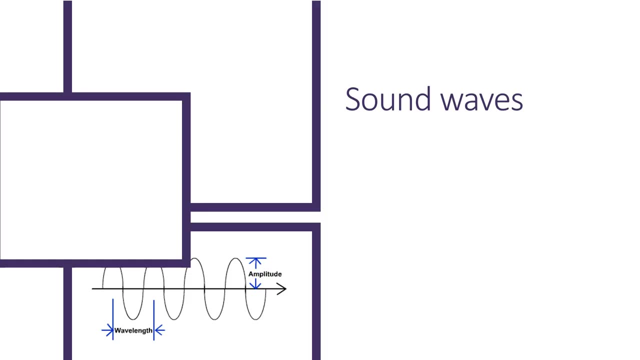 When we do output, we do the same thing in reverse. We take the digital values inside the computer and turn them into analogue outputs, And a very good example would be this: Sound waves are analogue measurements. We looked at how we can turn those smooth analogue signals into numbers inside the computer. 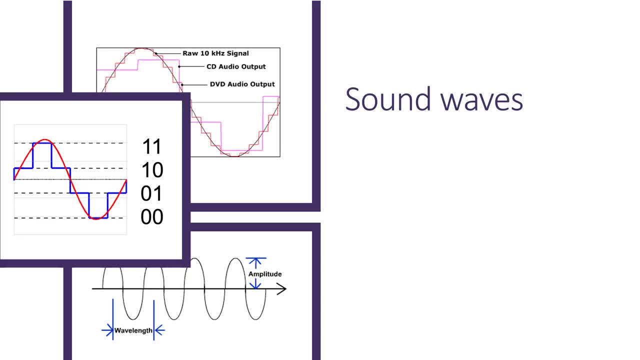 And it works in the other direction when we're talking about outputting sound. The digital numbers inside the computer are converted back into numbers. They are converted back into a smooth analogue sound signal. The more accurately and the more frequently we can output that digital information, the more realistic and rich the sound will be. 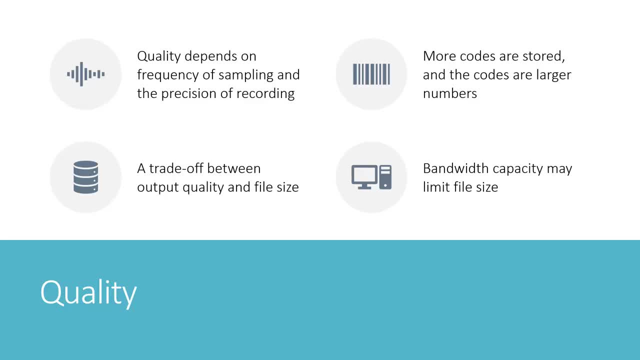 In general, there's a quality and capacity trade off. That is, signals such as sounds, which are more rich and realistic, require a greater number of digital codes, And the codes are larger numbers, So our quality is often limited either by the amount of storage that we have available. 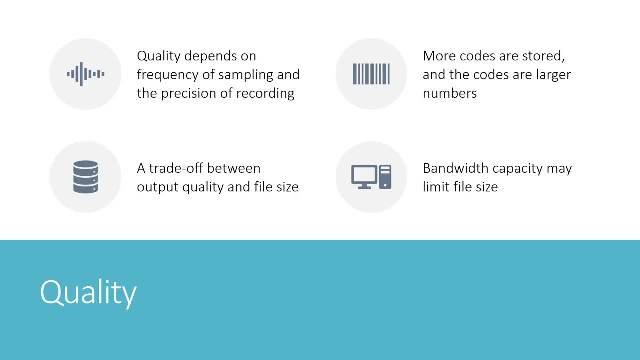 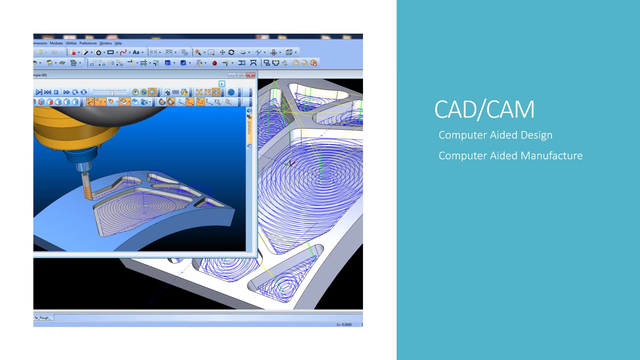 or increasingly in the modern world, by our bandwidth in transmitting the data, For instance as we download off the Internet. I want to briefly talk about another form of output, which is CAD-CAM, which is linked to the use of 3D printers. 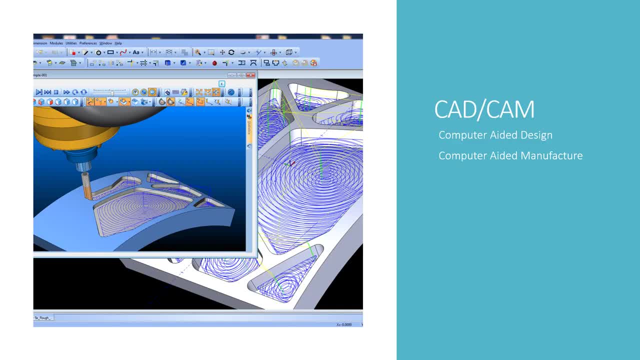 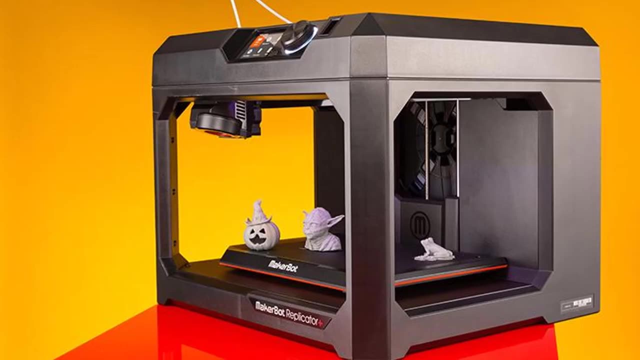 That is, we can design 3D solid devices on the computer, make our design, test our design without ever creating any real objects, And then we can output those devices using a 3D printer, And a 3D printer will spray or glue together some kind of solid matter. 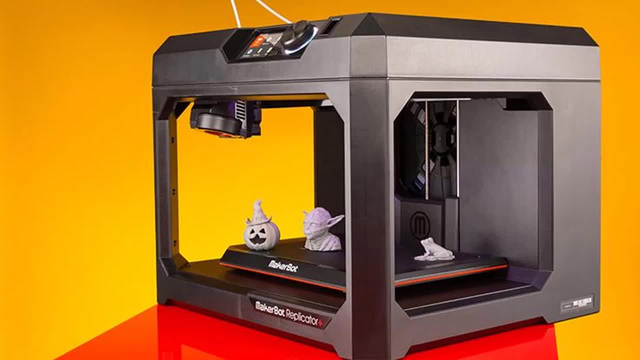 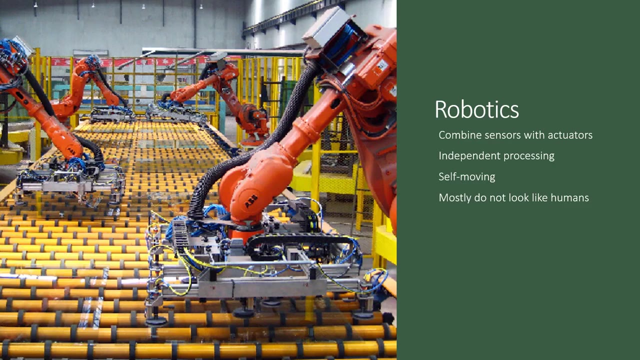 It might be a resin or a plastic, It could even be metal, And by sticking that together, actual 3D objects are output. We can also use a 3D printer. We can use a 3D printer. We can also combine input sensors with a sort of output device called an actuator. 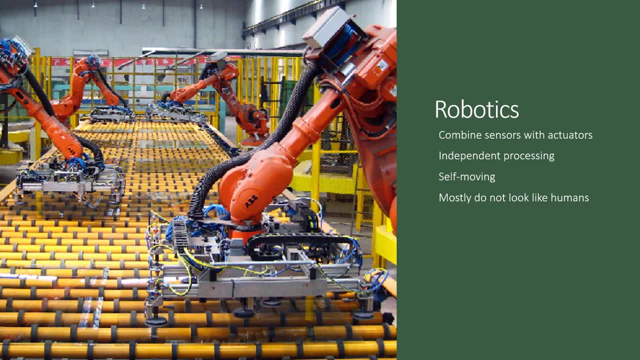 And an actuator will move, for instance, a robot around, And by combining sensors and actuators you can create some kind of robotic system. Most robots don't look like humans- These are examples of robots in a factory- But they can work automatically. 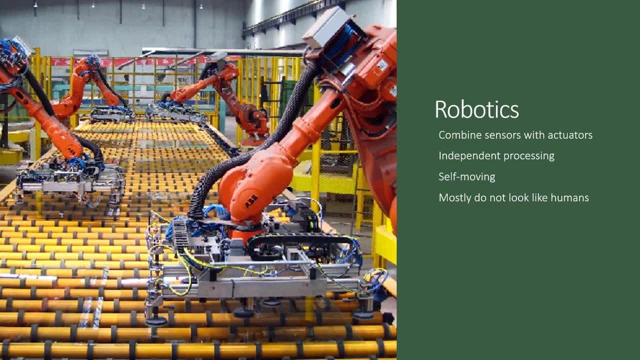 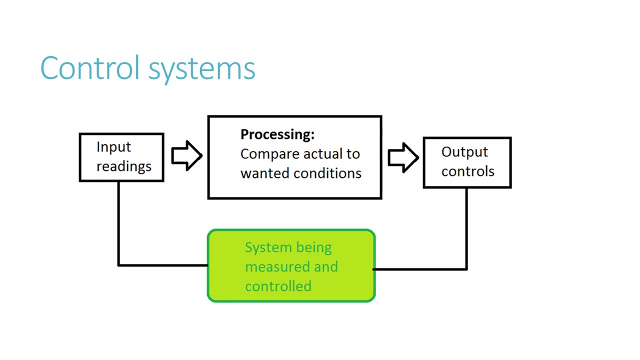 Without a human controlling them. There would be humans around to make sure that nothing's gone wrong, But the robots can do a lot of the work without anybody having to step in. Robotics is an example of what we call a control system, And there are lots of other kinds of control systems. 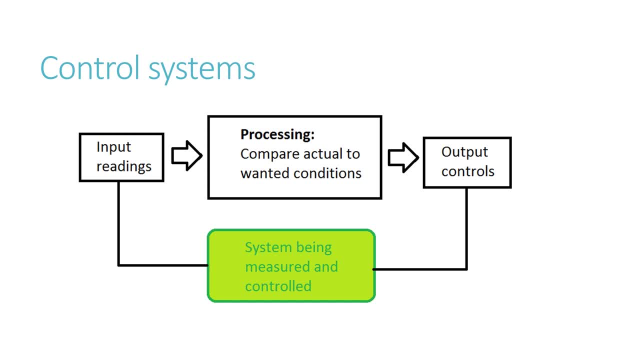 For example, let's imagine a bakery. There's a computer system that's controlling the temperature of the baking ovens. The system must have some kind of input so that the computer can tell how warm the oven has got. Inside the processor there is some sort of standard of how warm we want the oven to be.